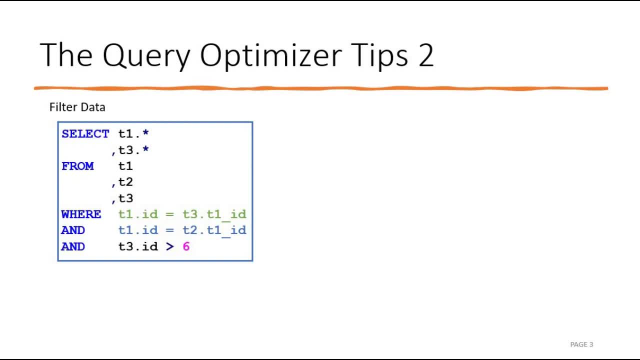 So let's see, we have another query where we want to fetch the column from the t1 table, t2 table and t3 table. So we can do a little better with document. We are going to show that the data is right, So write the query with document. 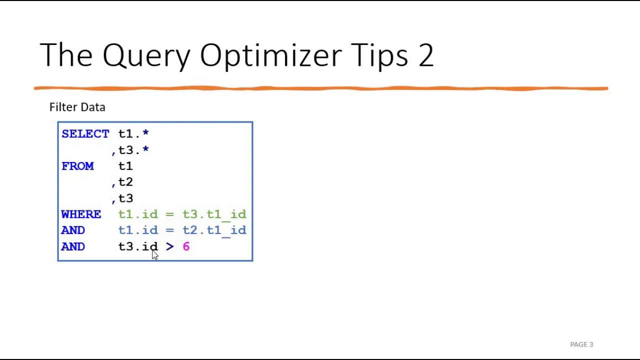 And if we have any info about t2, t3, i1, id, etc. for example, Then we will explain. this function is the QA function και test function created with document Iq Period. The 이제 sensations change and will lead to action errors again. So let's try it. You will see Now if what we do is we are getting results. you will say: what is our action error here, The activity here we are now doing? what I want to see is there is a leftover column and if a anytime we get an error here, then these cases will be loaded. 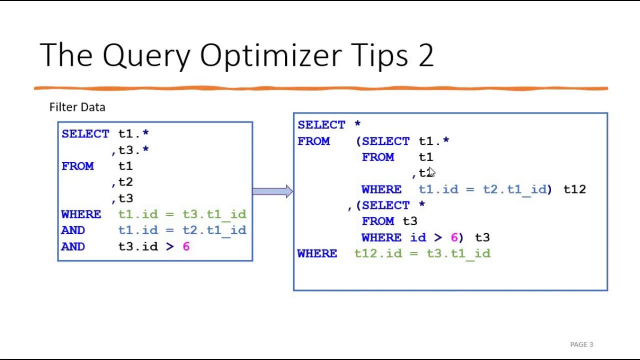 So we will try pop back that and test it what we have done. we have write two statement here. So the first is select statement fetching all the data from the T1, because here in the select statement we are, we need T1 data. 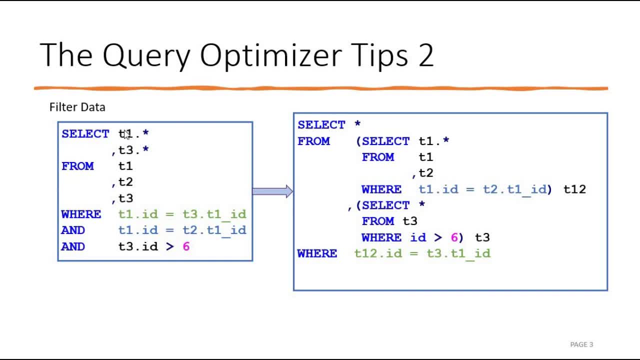 and T3 columns. So T1 columns and T3 columns. so that is why we have fetching here from the all the columns from the T1 table. So what we have done here- T1 and T2, we have. 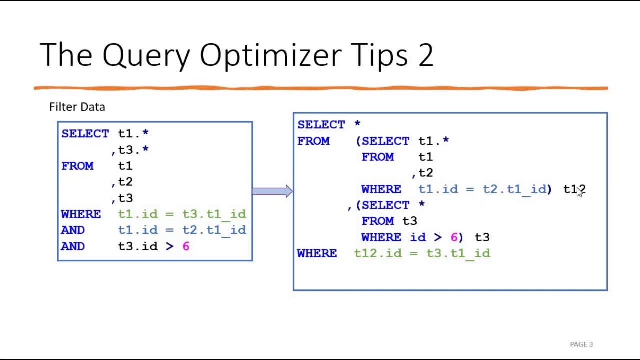 make a join condition here and we have just given alias here and another select statement from the T3 tables where we have mentioned the ID is greater than 6 here. So in this, in the select statement, we are fetching only those records which are greater than 6.. So 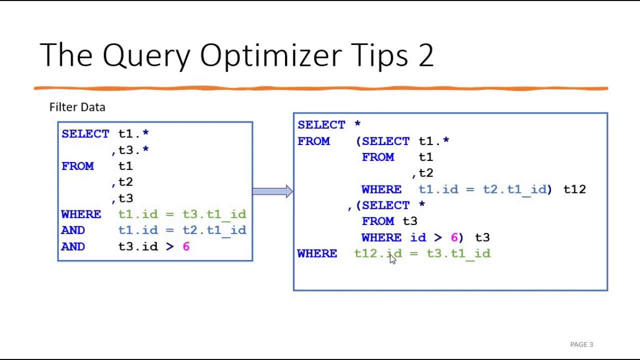 now in the upper select statement we have joined with this T12 ID and T3 IDs, So this way it will improve the performance of a select statement. So we do not need to fetch the all data- unnecessary data. We. 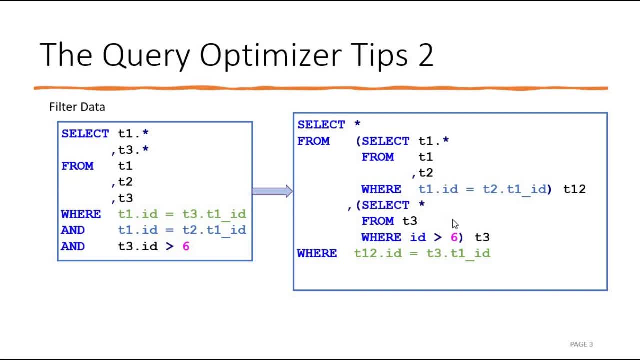 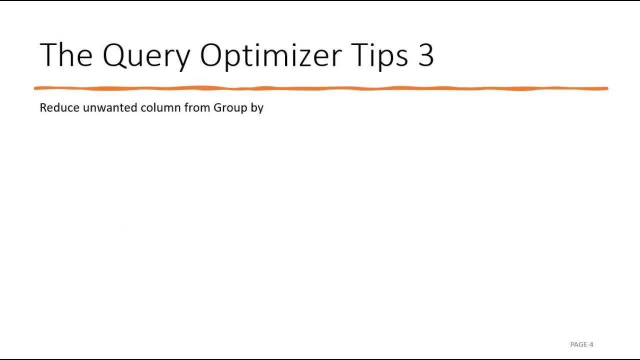 can filter out at the initial time itself when we are fetching the data from the select statement. Second example: how we can modify the existing SQL. Let us National SQL statement control, and which will improve. Let us see another example of how can we improve the performance of SQL statement. 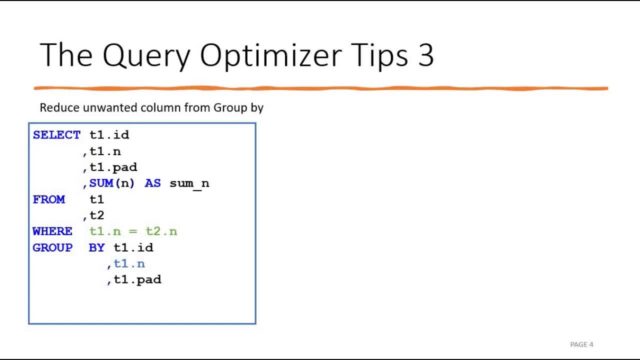 So here let us see, we have a select statement and here we are using a group like this. So we are fetching the column from the T1 ID, T1 end column and pad column and we are fetching the sum of it. So we are fetching the part and the 302 would be the points and 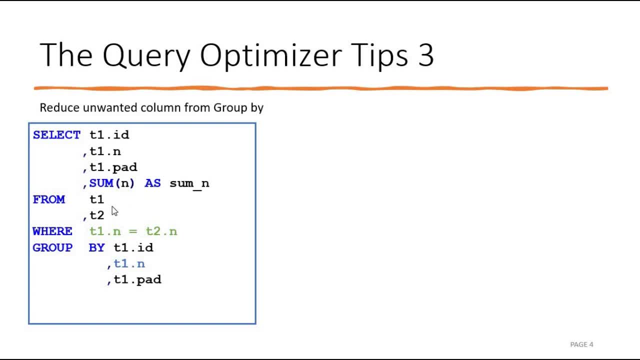 161, which gives us the column with the same quis. So we are here, we are creatinglo, acomplo the n column. ok, so here we are joining two tables, t1 and t2. we have added in where condition, and then, and here in the group by, we are mentioning id and pad these columns. how can we improve? 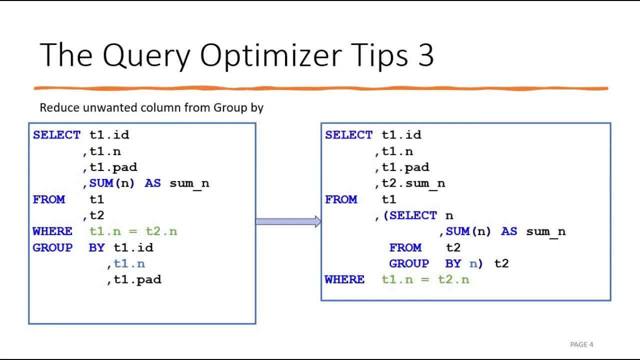 this select statement. let's see. so we can write this SQL statement in a different way which will improve the performance. so how can we do this, like in the inner query? first we will write a inner query which will have a limited columns in the group by, so here: 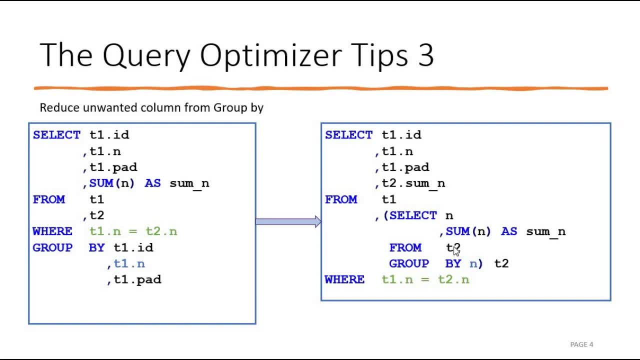 we are fetching the data from the t2- t2 table and here itself we are using a group by n, so only one column is used and we get the data which is required from the t2 tables. and now we are defining this t1 and t2 here in the where condition and in the select statement we are: 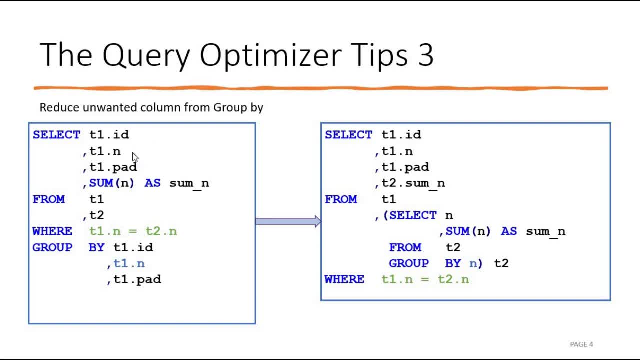 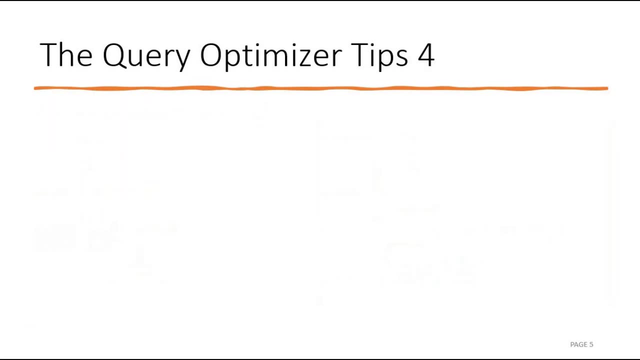 fetching all the columns which are required in the previous select statement. so this way we can improve the performance of a select statement, reduce unwanted column from the group by. let's see the another example: how can we tune the query? so let's say we have a select statement. I have seen so many queries in the production. also, people are writing. 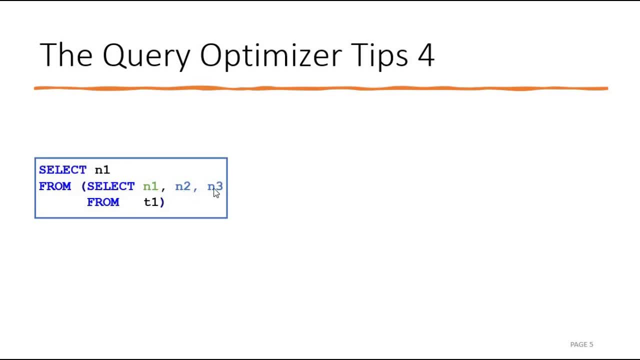 like this way: they are fetching the n1, n2, n3 columns from the t1 table and top of that they are using just single columns. how can we improve the performance? so we should use those column which are required. So here we can. So we can. 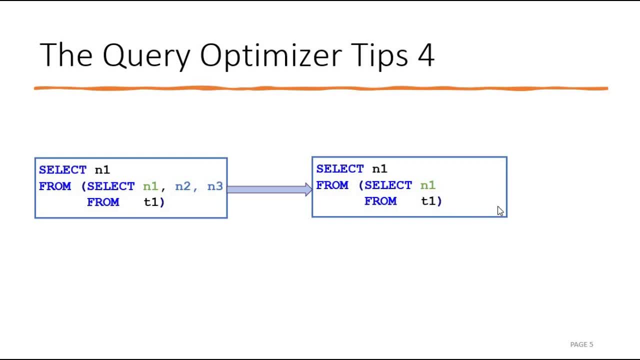 Write a select n1 from the t1, we can further improve this query. how can we do this? we just remove the inner query. we just use select n1 from the t1. so this way we can improve the performance of the select statement, reduce unnecessary column or expression from the 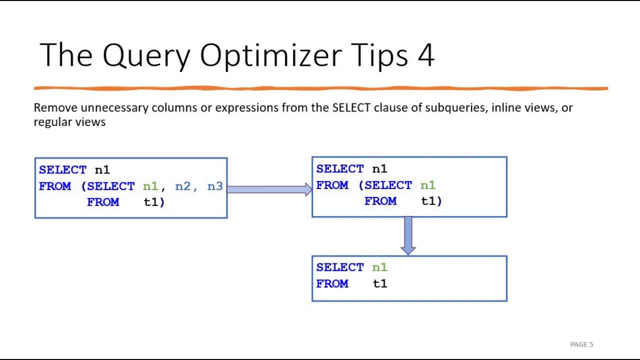 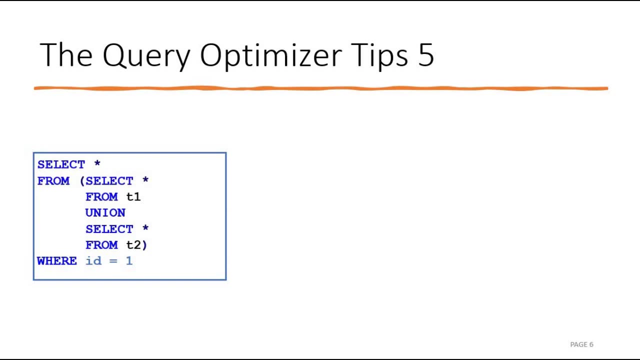 select clause or subquery, inline view or regular view. Let's see the another example. how can we improve the performance of a SQL statement? so let's say, here we have a select statement where we are fetching the data from t1 and t2 using union all and after that we are applying that we want the id data from id data, which. 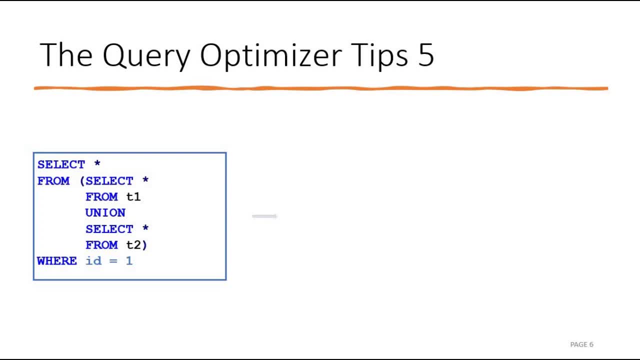 is equal to 1.. So how can we improve this? We can write this select statement in a different way to improve the performance of a SQL statement. So let's see how we can do this, so we can use a different way, like select star from. 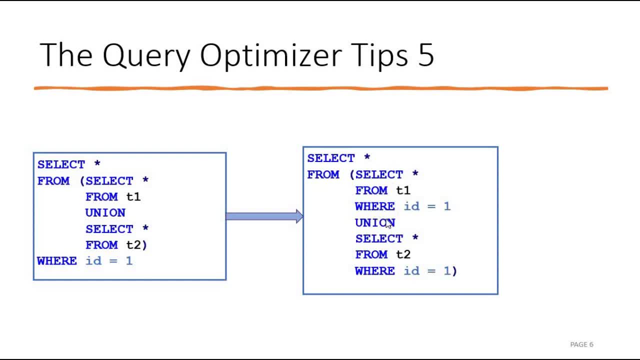 t1 in the union all only. we will add a where condition because after filtering in the first select statement, fetching all the records from t1 and t2, and then later on we are adding condition, like we need a data for id equal to 1 only. So what we can do here in the next selected statement. 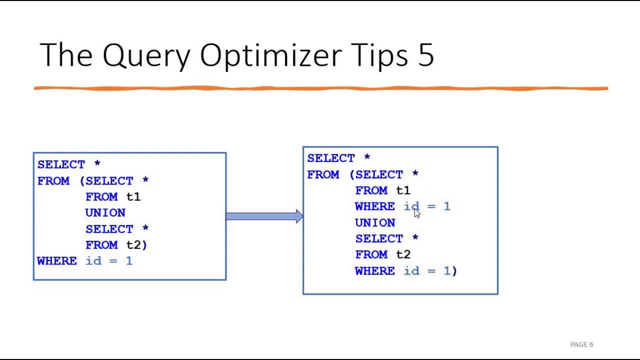 which will improve the performance of SQL statement. we will fetch the id, which will fetch the data from the t1 table where id equal to 1 at the initial time only. So we will add the where condition here in the for the t1 and t2 also, and then on top of. 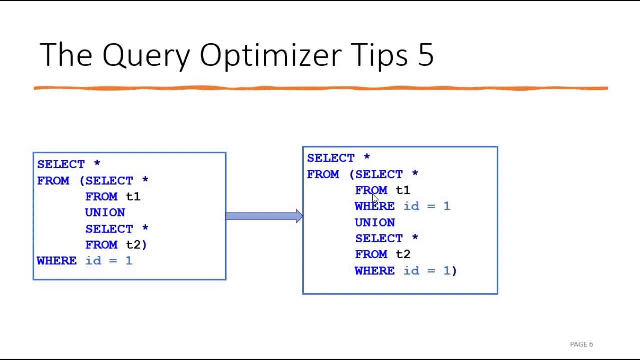 that we will fetch the select star from all the records, from t1 and t2.. So this way it will improve the performance. So we should. the purpose of this filter push down is to push restriction inside the view or inline view that can be merged.